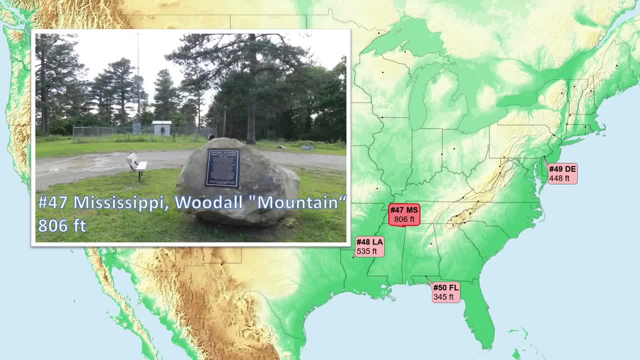 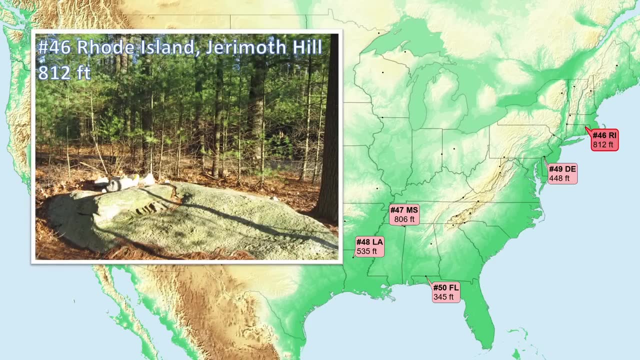 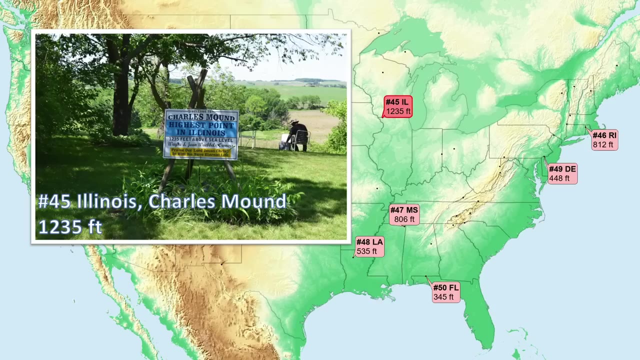 capped by more resistant rock, in this case sandstone, than the surrounding area. Number 46, Rhode Island, An attractive forest site with a big boulder comprising the high point location. Number 45, Illinois, Our first high point, over a thousand feet, the first inland state. And here we start. 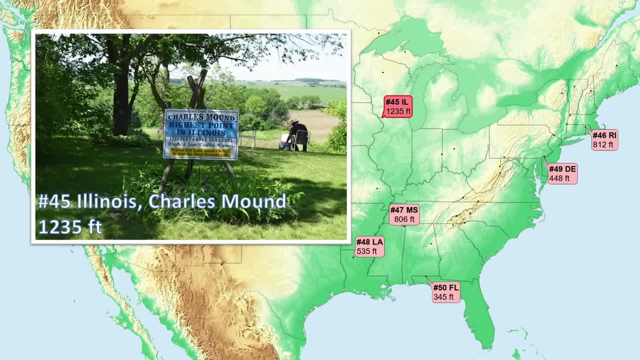 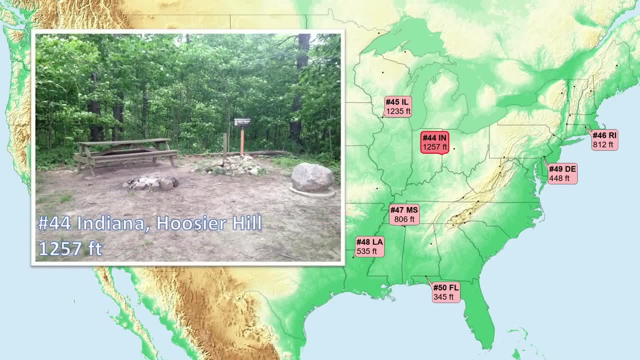 a streak of Midwestern states. This corner of Illinois is in the driftless area that avoided glacier erosion that flattened much of the surrounding Midwest. Number 44,, Indiana, Near the eastern edge of the state, glacial moraine deposits So that 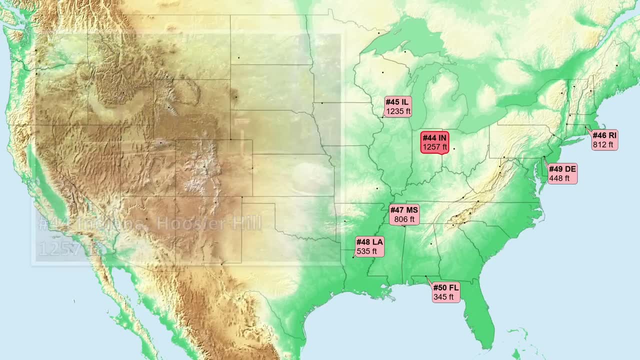 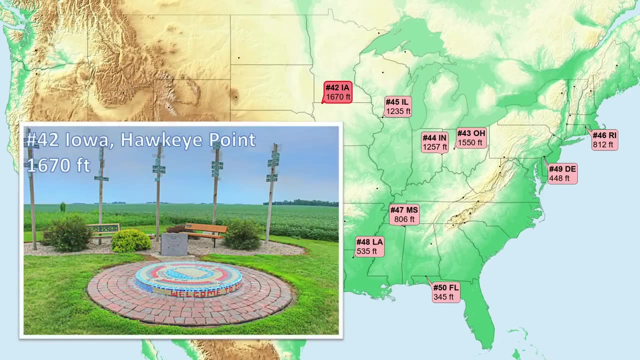 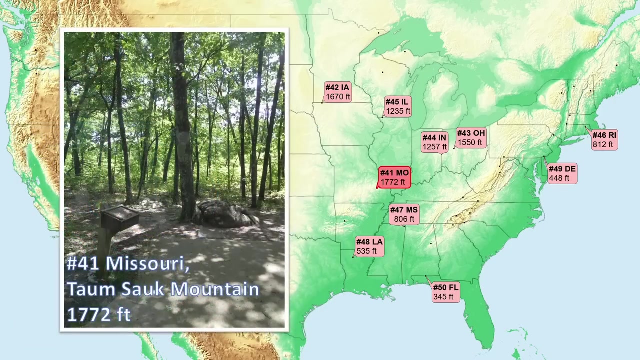 is piled up material left behind by the continental ice sheets. Number 43, Ohio, Also a moraine deposit. Number 42, Iowa: Another glacial moraine up at the northern edge of the state. 41 is Missouri. This high point is associated with very ancient volcanic activity that occurred well. 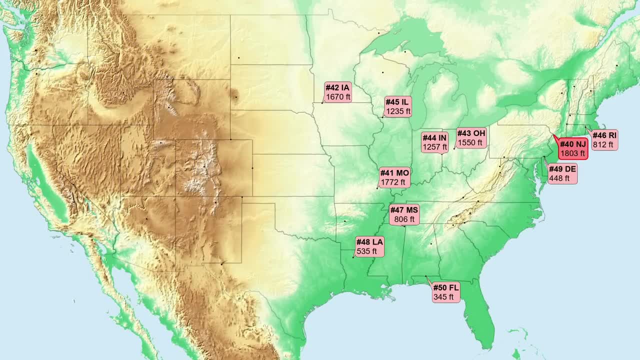 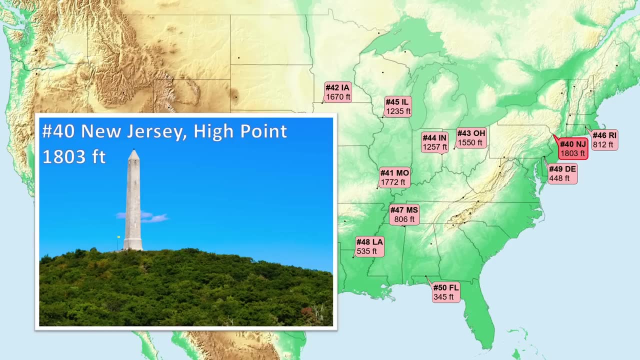 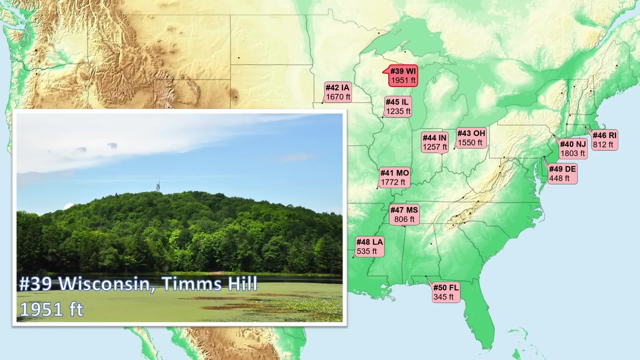 over a billion years ago. 40, New Jersey: Here, near the northernmost point of the state, is a sedimentary rock rich in quartz which is very resistant to weathering. 39, Wisconsin, On a thick accumulation of glacial debris over top Canadian Shield bedrock. 38, Michigan, A granitic rock peak. 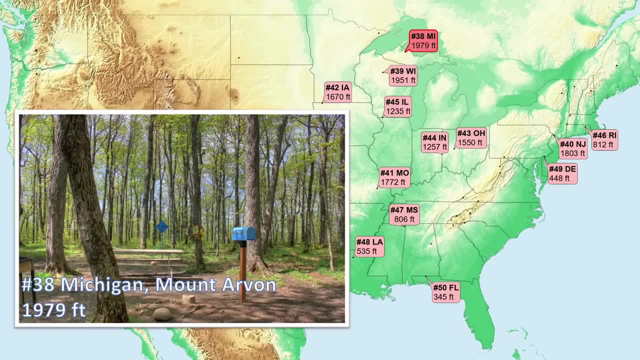 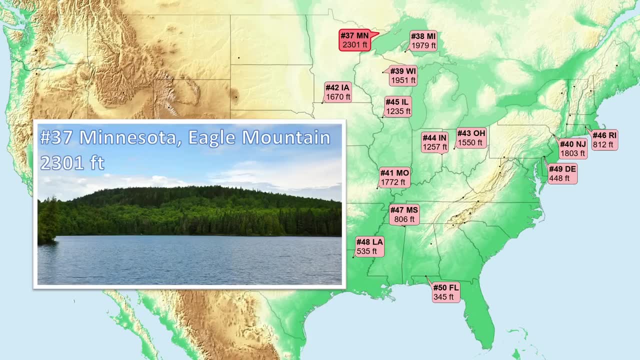 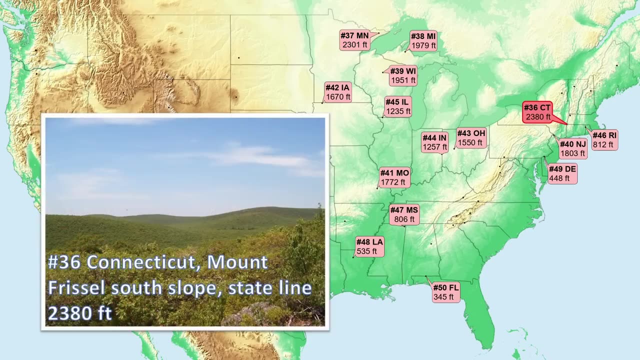 of the Canadian Shield, heavily sculpted by continental glaciations, with much terrain covered by glacial till. 37, Minnesota, First, over two thousand feet. Also a glacially sculpted granitic rock peak of the Canadian Shield. 36, Connecticut, On the state line on a 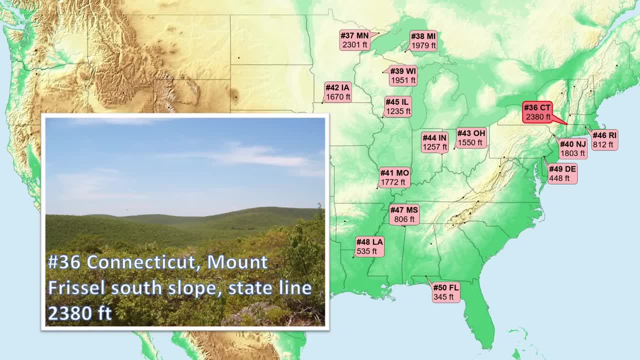 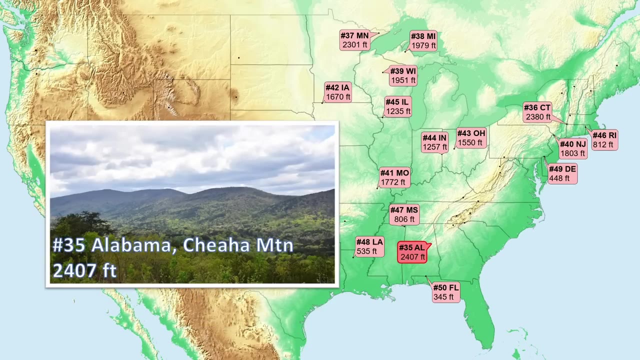 mountainside with its actual peak to the north, outside the state. this high point is composed of metamorphic rock. It is part of the Appalachians and thus associated with old North American plate collisions on the east side of the continent. 35, Alabama- Here meta sandstone and quartzite rock. 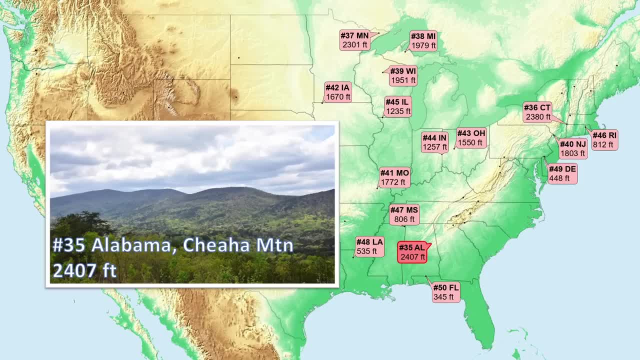 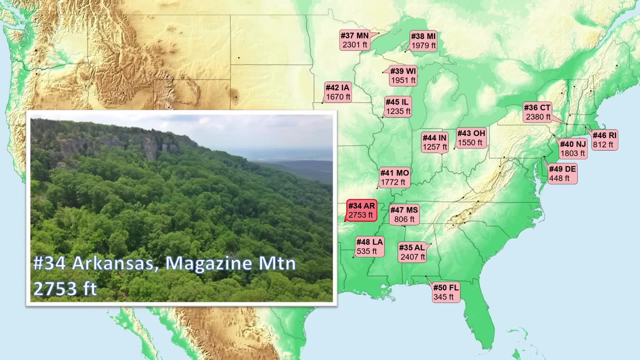 surface rocks have high erosional resistance, resulting in raised topography. This is the high point closest to the mean elevation of the US. It's less than 100 feet below that mean. 34,. Arkansas, A sandstone, capped plateau high point associated with a mountain system that 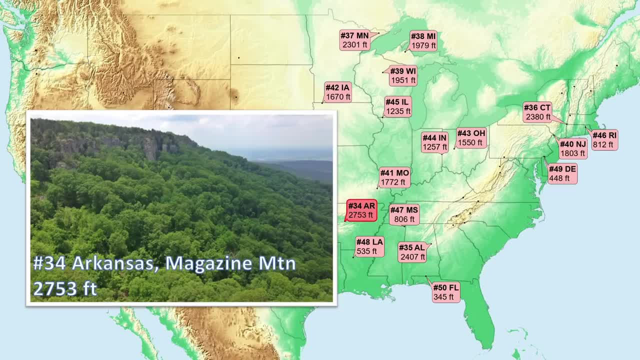 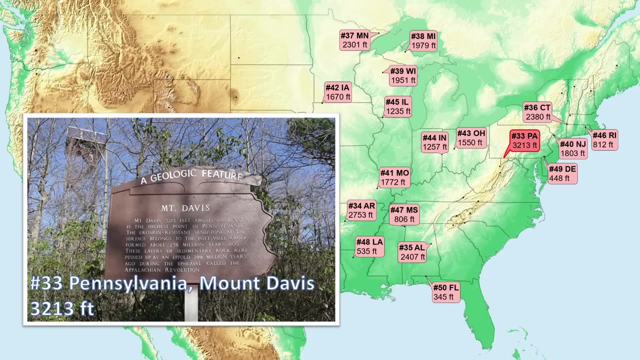 trends mostly east-west. unlike most US ranges, It's related to ancient North and South American plate collision and we're up to an elevation now where only about five percent of the US population lives above 33,. Pennsylvania First high point, over three thousand feet, situated atop a long 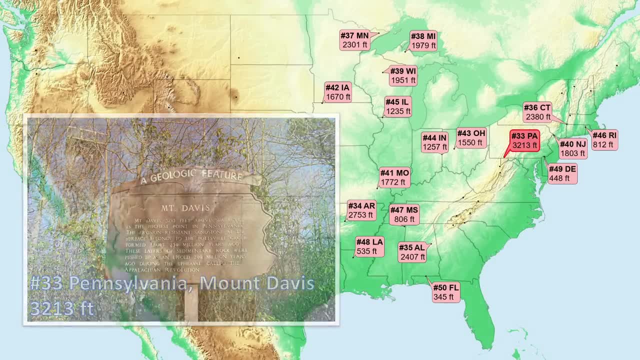 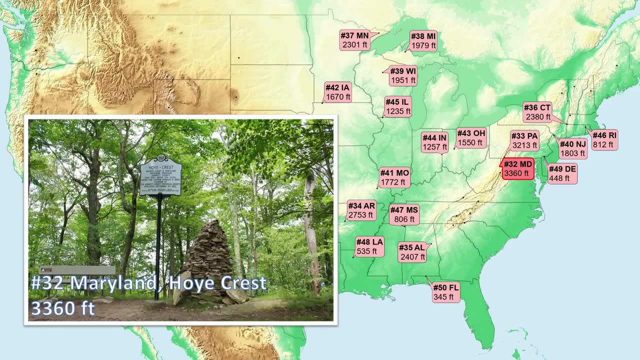 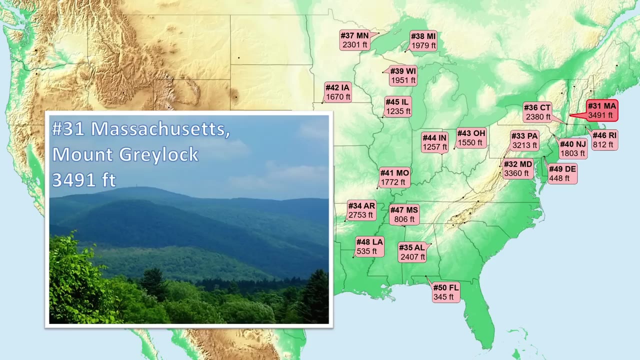 resistant sandstone ridge of the Appalachian Mountains 32, Maryland. This site is close to the border with West Virginia, atop another long resistant ridge of the Appalachians 31,, Massachusetts. Here in the northern Appalachians, rocks consist of relatively high grade metamorphic and igneous rocks with great 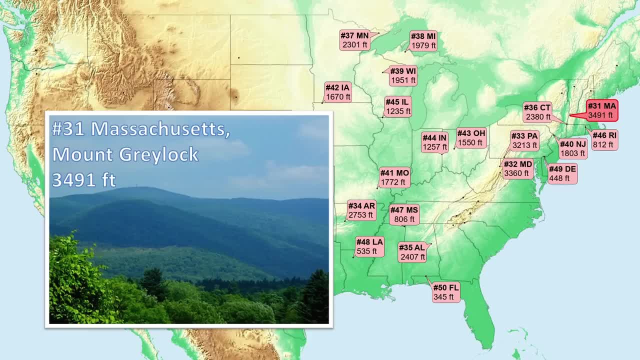 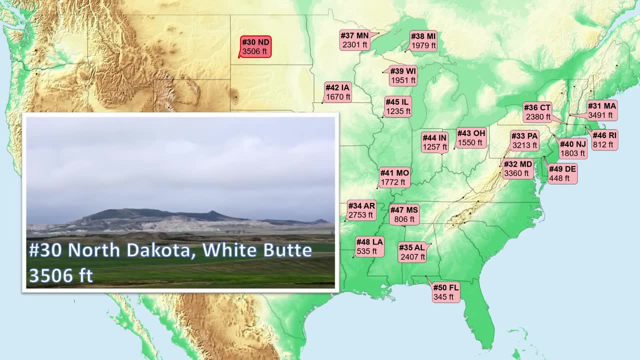 resistance to weathering and thus rise above adjacent areas of lower grade metamorphic and sedimentary rock. 30, North Dakota, Our first western state. Here, a sandstone, capped plateau, capped peak, is within heavily eroded sedimentary rocks of this upper Great Plains region. 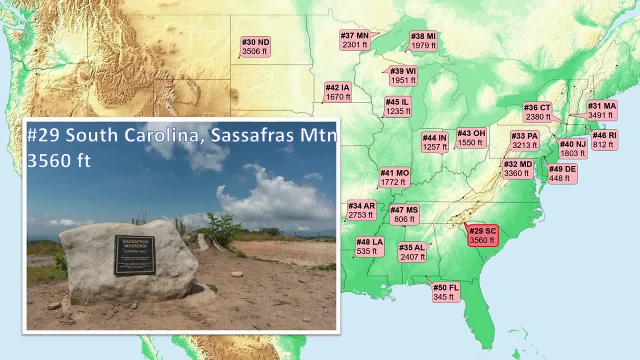 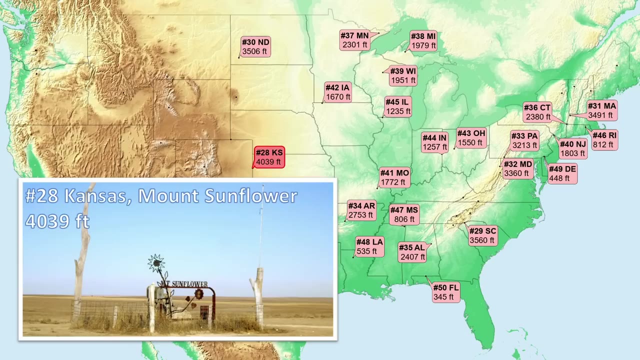 29,, South Carolina. Back to the Appalachians and up against the North Carolina boundary, granite that originally formed this mountain has metamorphosed into gneiss, the highest grade metamorphic rock, type 28,. Kansas First peak, over four thousand feet. 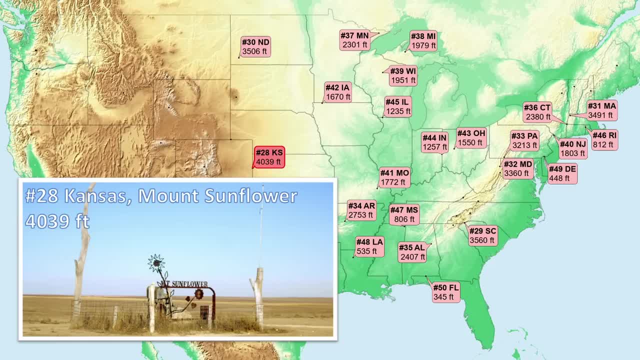 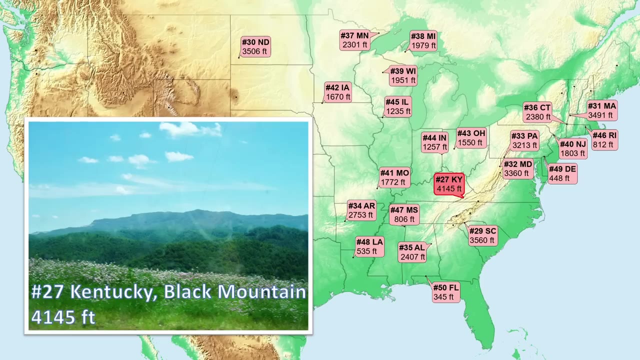 near the border of Colorado. Not a prominent peak at all, just have a state with a dominant topographic gradient, from central lowlands to high plains, going east to west, which you can see on this relief map 27,, Kentucky, Back to the Appalachians, again near the Virginia border. 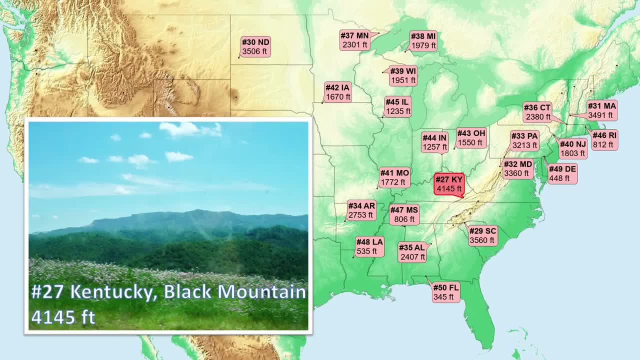 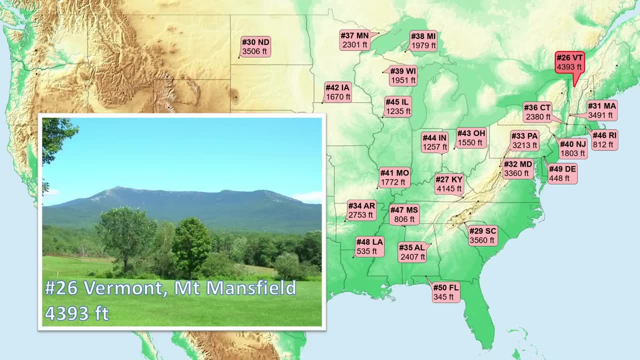 another sedimentary rock ridge here, quite rich in coal 26,. Vermont. Back in moderately high grade metamorphics of the northern Appalachians. at this high point, that still has remnants of alpine tundra. At this halfway point, higher terrain still remains across the country. 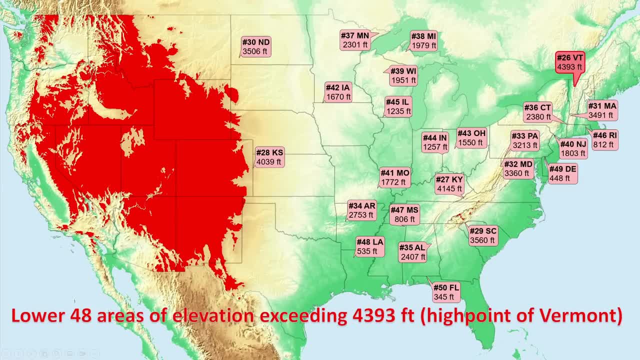 There's a few more high peaks in the northern Appalachians. It's hard to make out these very small areas. There are a few larger peak areas in the southern Appalachians, but look how much terrain in the west still lies above our middle-ranked Vermont high point. Of course, 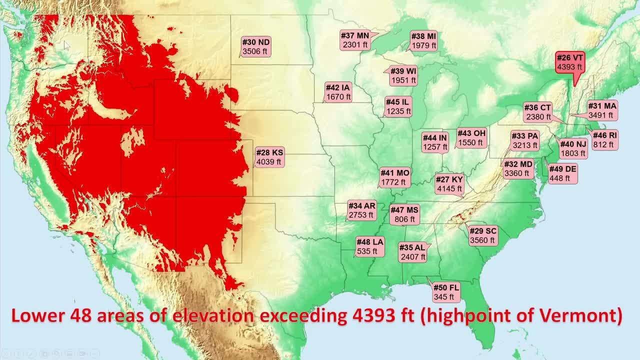 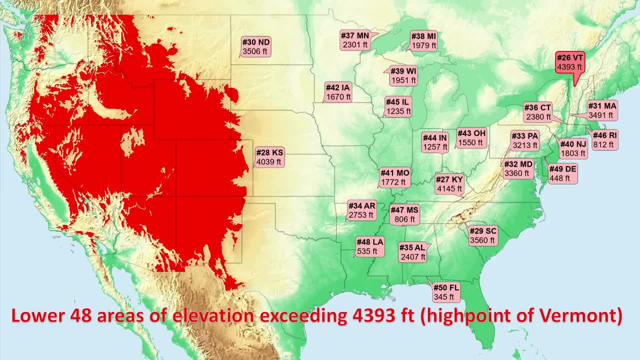 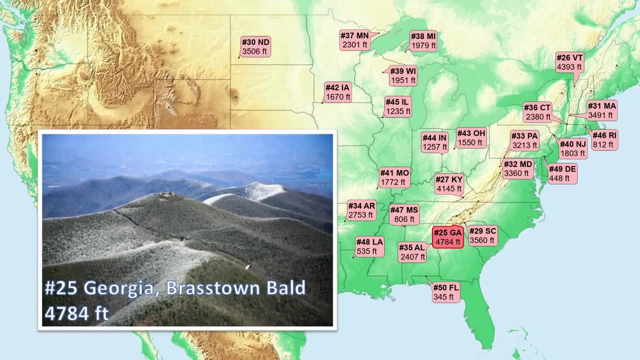 But also high broad areas too, like the Colorado Plateau and much of the basin and range region 25, Georgia, At the north end of the state, in the Appalachians, where thrust faults expose a variety of resistant rocks once buried deeply in these mountains. 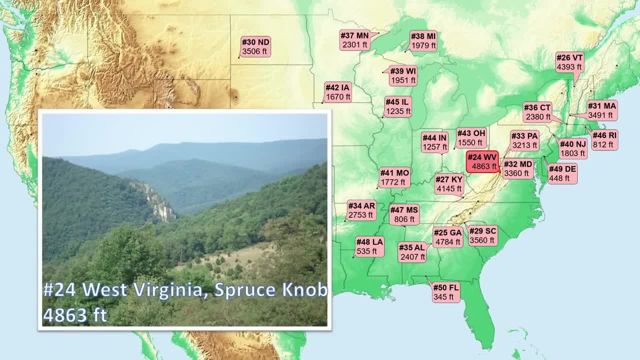 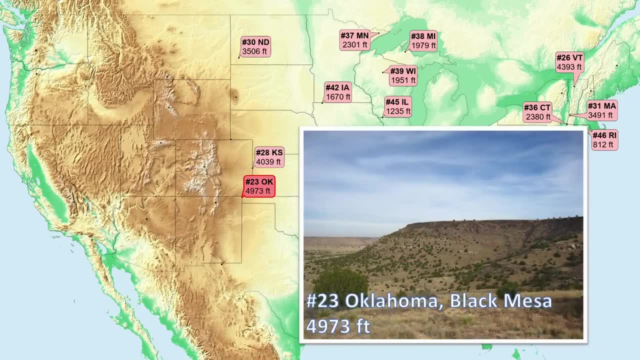 24, West Virginia, Part of another one of these long major sedimentary rock ridges of the central Appalachians. 25, Oklahoma. Number 23, Oklahoma. Up in the northwest corner of the state, mesas are flat-topped hills left. 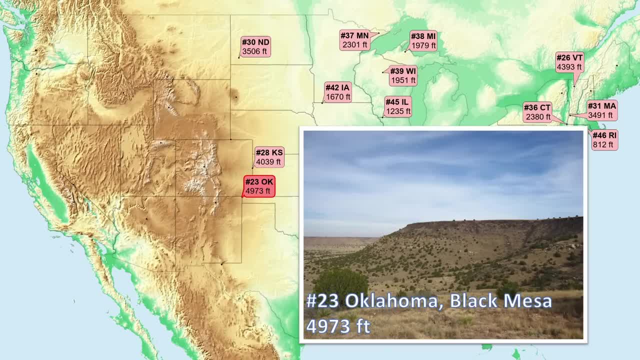 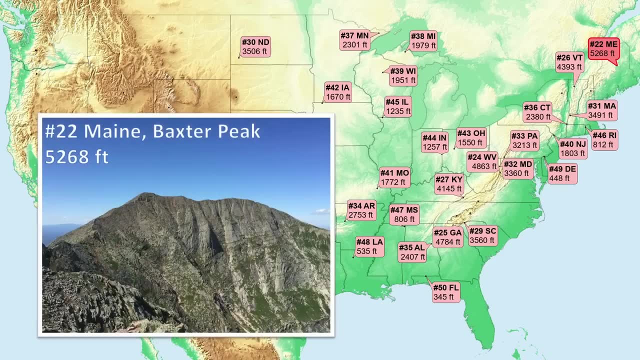 by erosion around horizontal rock layering. This high point, mesa, is capped by a basalt lava flow, less than 5 million years old, from a volcano located in Colorado, 26, Colorado, Number 22, Maine, First peak, over 5,000 feet. this mountain formed from a large granite intrusion. 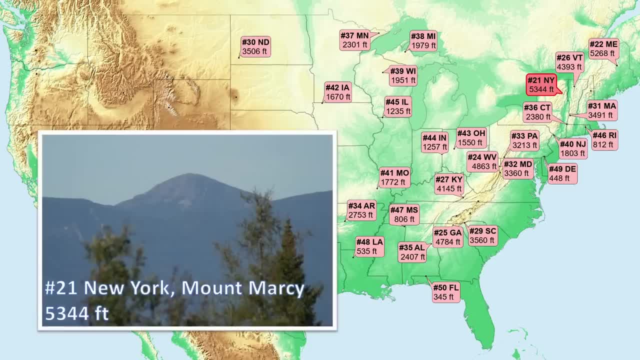 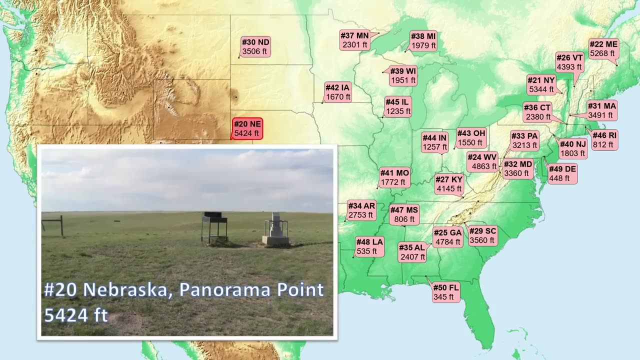 eroded to the surface. 27, Colorado, 28, Colorado. Number 21, New York- Another granitic massive peak here in the heart of the Adirondack High Peaks region. Number 20, Nebraska: Very similar to Kansas, with a high point located almost on the Colorado border. 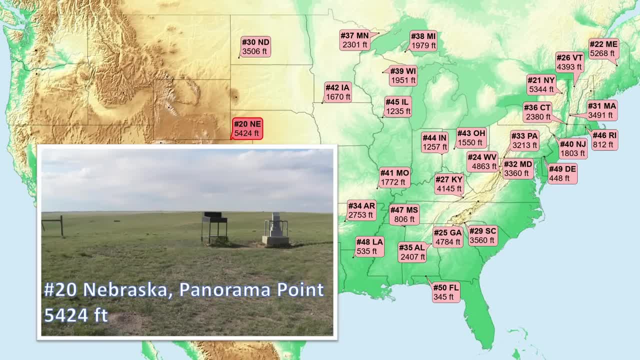 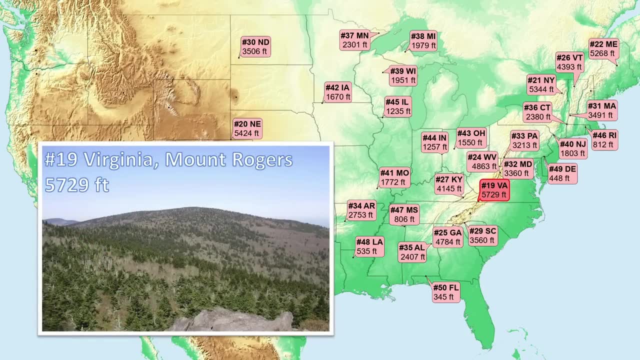 in a western corner of the state, terminating the state's long east-west elevational gradient, Number 19, Virginia. Tucked in the corner of the state, this mountain contains a set of rocks that is about 30 percent sedimentary and 70 percent volcanic, With a volcanic. 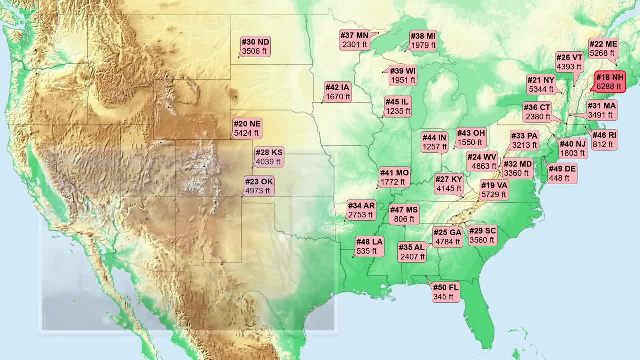 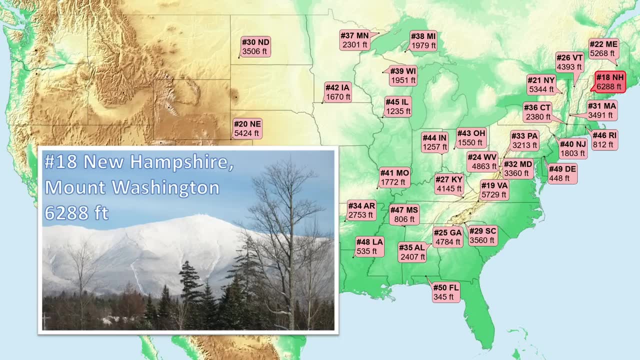 eruption. this rock, positioned near the upper edge of the state, is gigantic, forming the hard resistant rock that holds up the peak Number 18, New Hampshire. This high point is most famous for its long held world record for the highest measured wind speed not within a tornado or a tropical cyclone: an astonishing 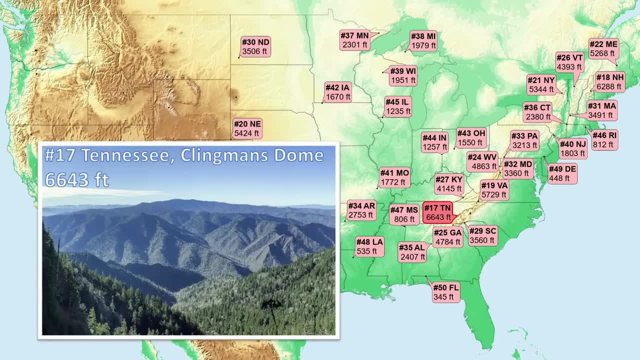 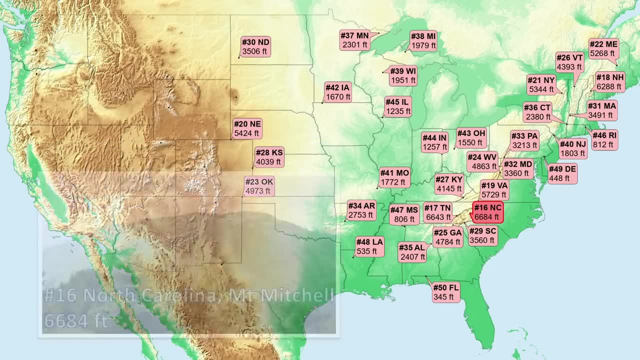 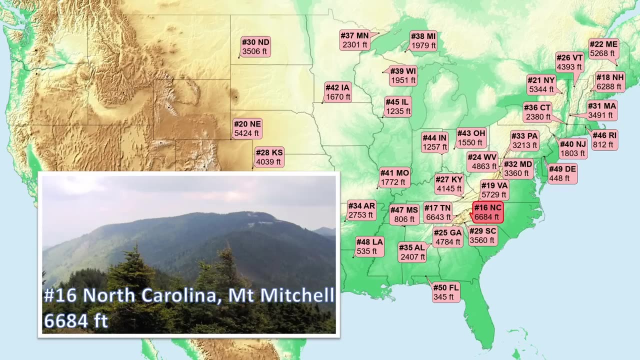 231 mph, Number 17,, Tennessee. Near the eastern edge of the state. this Appalachian peak consists of a variety of hard metasedimentary rocks east of the Mississippi. This impressive eastern mountain formed during the pre-Cambrian when. 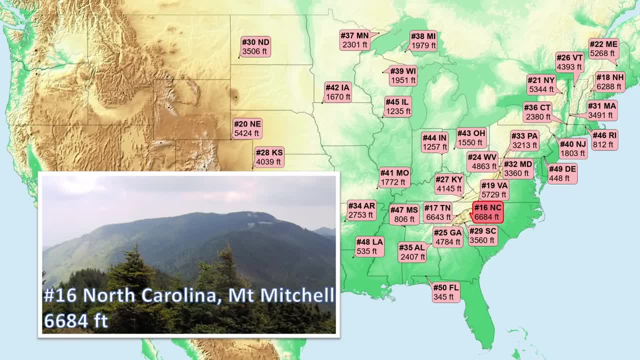 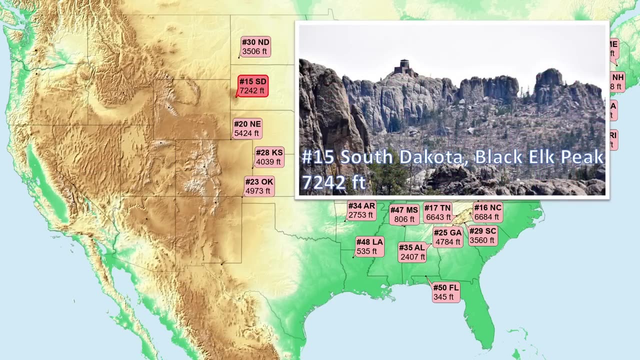 marine deposits were metamorphosed into nice and other high-grade metamorphic rocks. These rocks were later uplifted during an immense continental collision. that was part of the great geological mountain-forming events that created the long Appalachian mountain chain. Number 15, South Dakota: Only western states. now for the rest of our countdown. 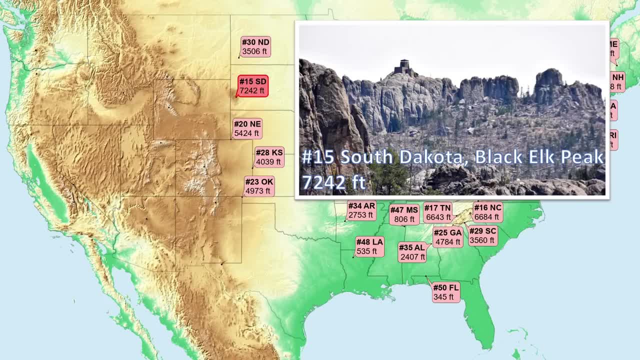 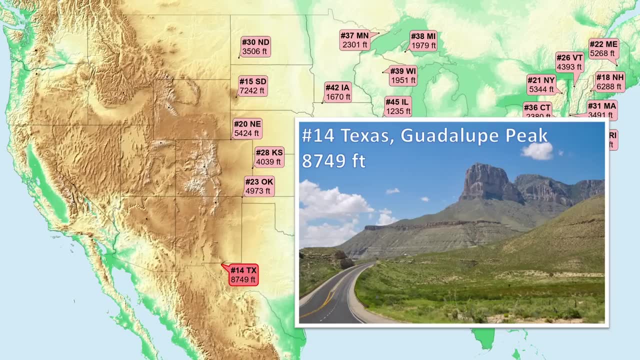 This peak is part of a granite dome uplifted to form the interesting Black Hills region, the same granite seen at Mount Rushmore, Number 14, Texas. We're now at a part of our series where elevations increase more quickly, with this being the first of three in a row with over 1,000 foot increase from the previous state. 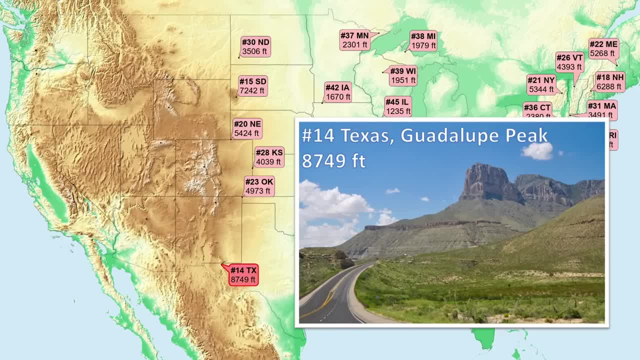 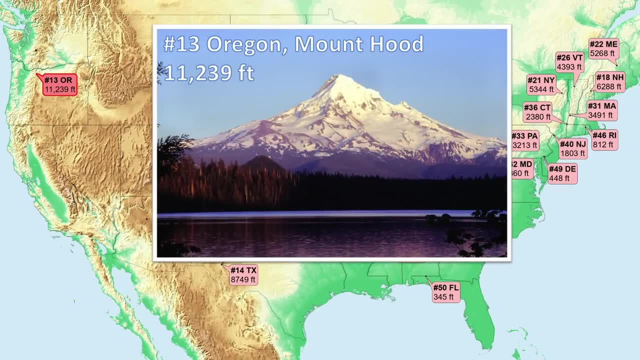 Faulting 20 to 30 million years ago uplifted a large, beautifully preserved fossil reef to form this limestone. high point Number 13,, Oregon, First, over 10,000 feet and a beautiful example of a strata volcano, Part of the Cascade Volcanic. 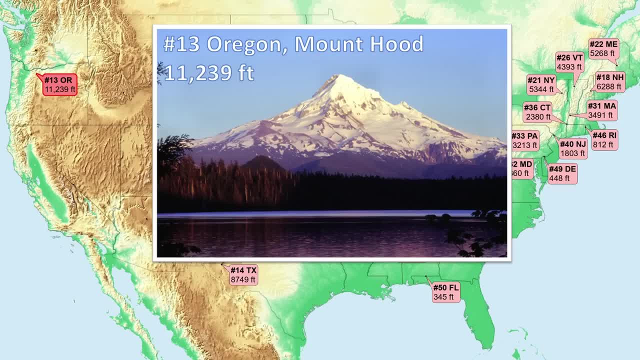 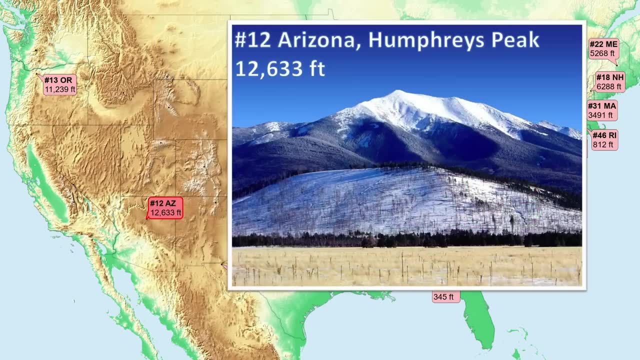 Arc formed from the tectonic subduction zone along most of the US west coast. It is still active. Most recent eruption 1865.. Number 12, Arizona, Now an interior state, strata volcano, this one being extinct and highly eroded. Its last eruption occurred about 400,000 years ago. 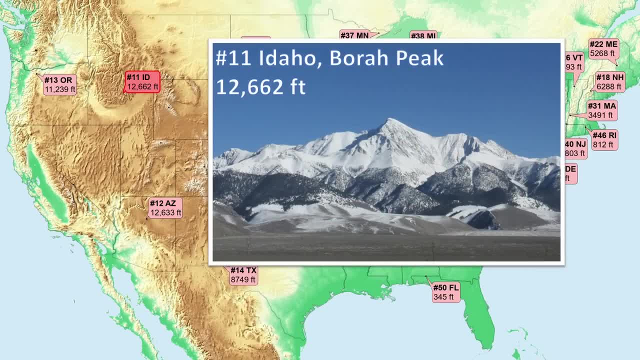 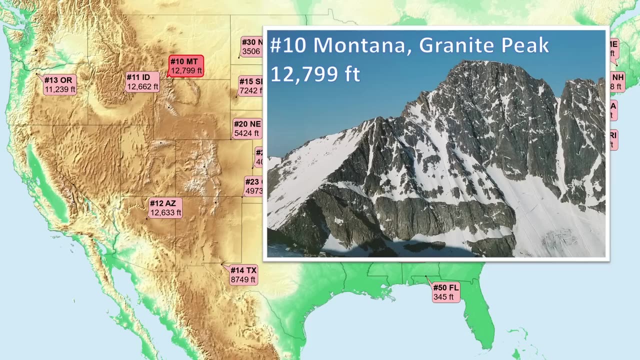 Number 11, Idaho. The steeply tilting limestone layers of this high point were, incredibly, raised by about a foot just in 19.. 83 by a magnitude 6.9. earthquake. Number 10, Montana. Near the state's southern border in the Beartooth Mountains, this peak is an impressive 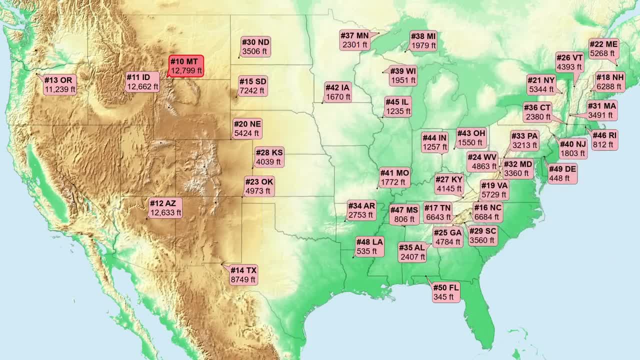 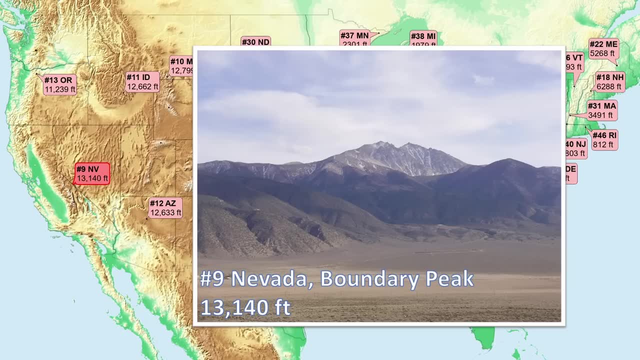 complex of granite and gneiss more than 2 billion years old, Number 9, Nevada. It's actually a subpeak to a higher summit- less than one mile away in California, Granitic, and part of the White Mountains, which is a fault block mountain range formed by 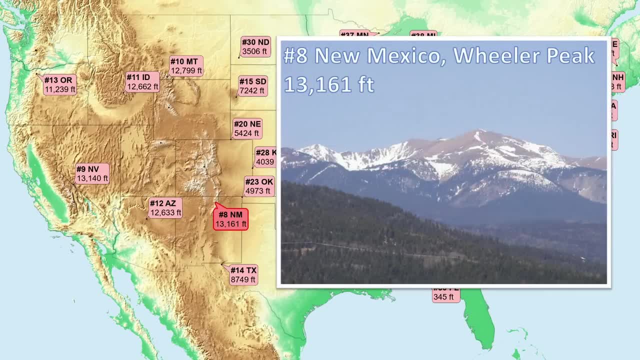 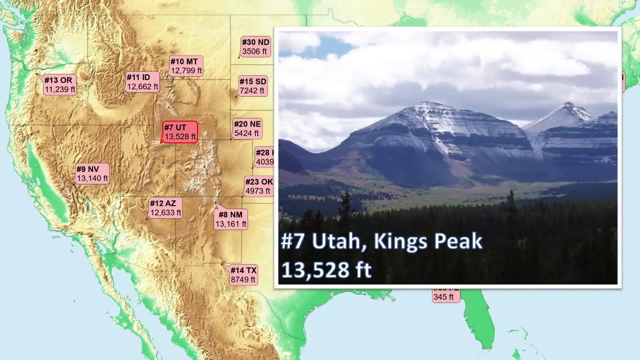 extensional tectonics. Number 8, New Mexico: In the northern part of the state, In the southernmost sub-range of the Rocky Mountains, this peak is made up of uplifted high-grade metamorphics. Number 7, Utah: Uplifted metasedimentary rocks in the Uinta sub-range of the Rockies. that is unusual as the highest range in the contiguous US. 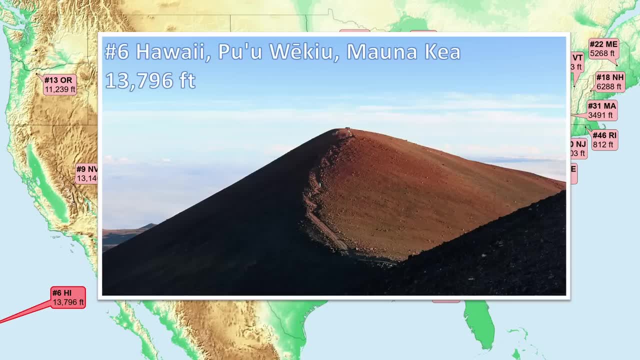 oriented in the east-west direction. Number 6, Hawaii: An extraordinary high point of an enormous young shield volcano formed from hotspot volcanism way out in the Pacific. It's the tallest mountain on our planet when measured from its underwater view. Number 7, Utah: Uplifted metasedimentary rocks in the Uinta sub-range of the Rockies. that is unusual as the highest range in the contiguous US. oriented in the east-west direction. 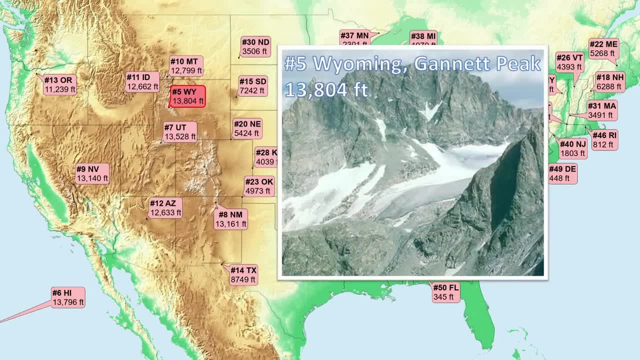 It's the tallest mountain on our planet when measured from its underwater base Number 5, Wyoming. Only an eight-foot step up to this inland state high point in the beautiful Wind River Range, The continental divide follows the crest of this primarily granitic high-range. Number 4, Washington, An imposing glaciated stratovolcano in the Cascade Range of the Pacific Northwest and the tallest peak of the Cascade volcanic arc. This stratovolcano has a high probability of eruption in the near future and is considered one of the world's most dangerous volcanoes. 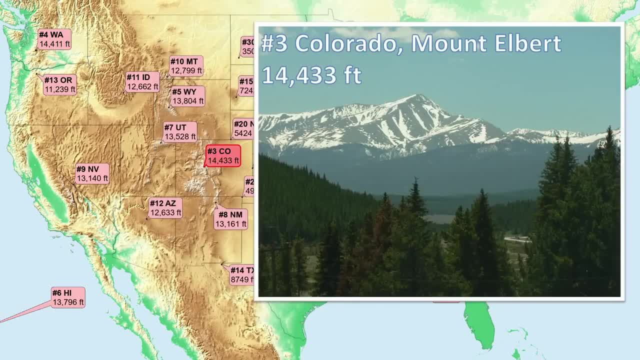 3. Colorado, A mountain composed largely of quartzite with a summit ridge of pre-Cambrian metamorphics. This is the highest high point of the Rocky Mountains, the largest mountain system of North America. The Rockies were formed by contractional tectonics when a number of plates slid beneath the North American plate. 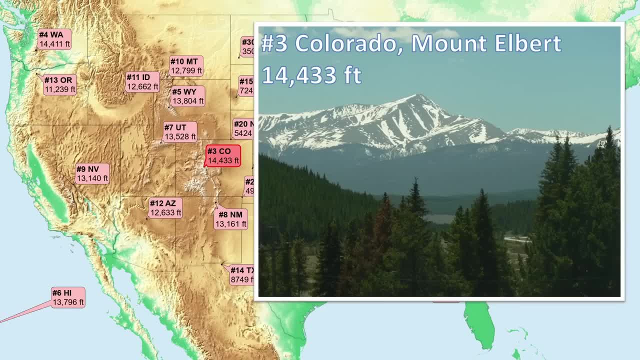 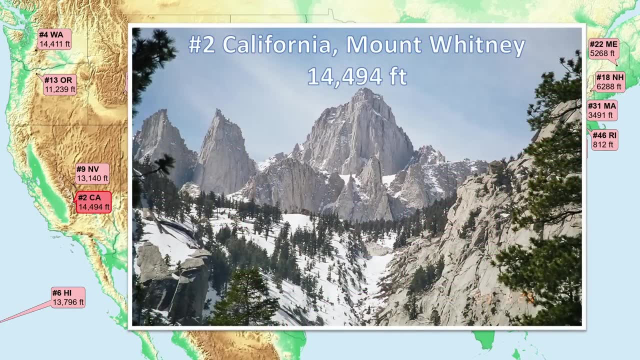 at a shallow angle of subduction, resulting in a broad belt of thrusted and folded mountain ranges. 2. California: Like the previous two peaks, another 14er, This one being the highest mountain of the contiguous US. The uplifted granite forming this peak is part of the Sierra Nevada Bathliff. 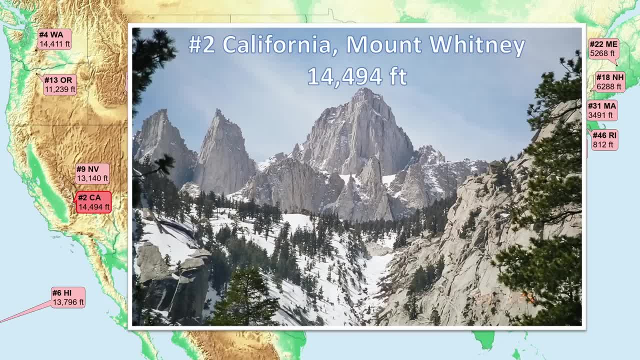 a huge mass of solidified molten rock originating from subduction. The east mountain slope is far steeper than the west, because the entire range is made up of a slightly tilted fault block. So this is, then, a near final map of high points of the United States. 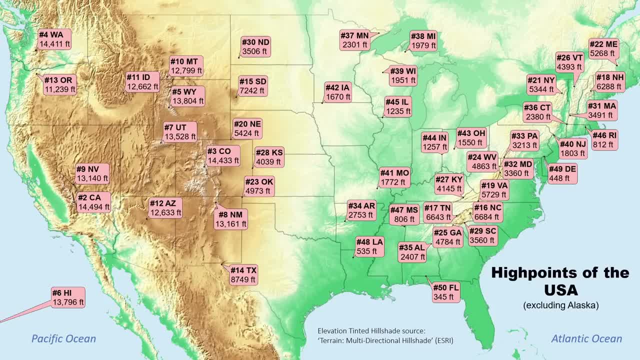 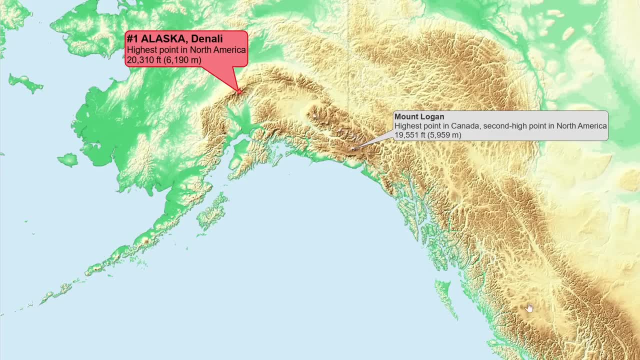 However, there is one more monster of a peak we can't forget about. Let's zoom in. Let's zoom up to Alaska. By far the biggest vertical step up in our sequence. At a staggering 20,310 feet, the world-famous Denali is the highest peak of the entire continent. 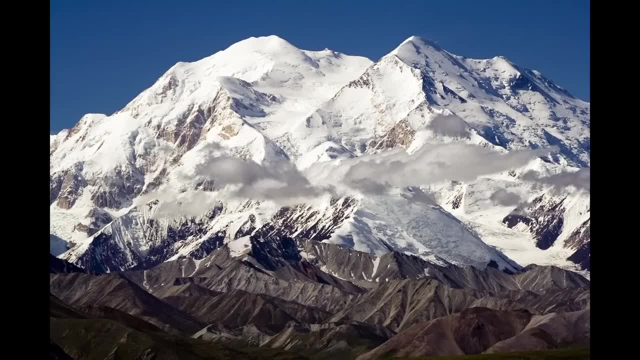 Denali is a granitic pluton that has been lifted by tectonic pressures from the subduction of the Pacific plate beneath the North American plate in this most geologically active part of the country. As it has been lifted, sedimentary material above and around the mountain was stripped away by erosion. 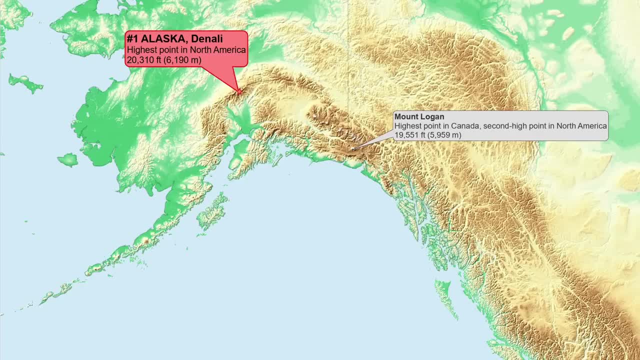 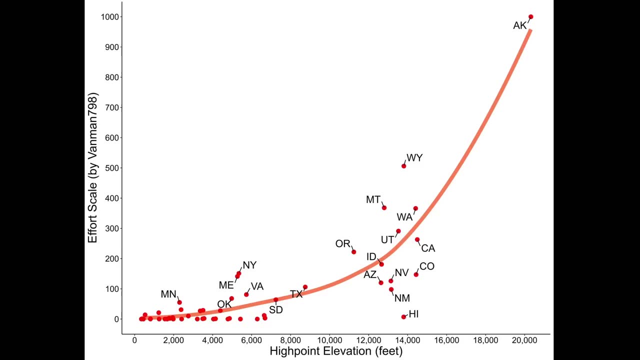 especially by glacial activity. Canada also has an extraordinary high mountain in this same tectonic region called Mount Logan. An interesting question is whether there is a relation between high point height and difficulty to climb. I found a nice effort scale analysis by Vaman798, see video text for sources- and there is a pretty good fit.